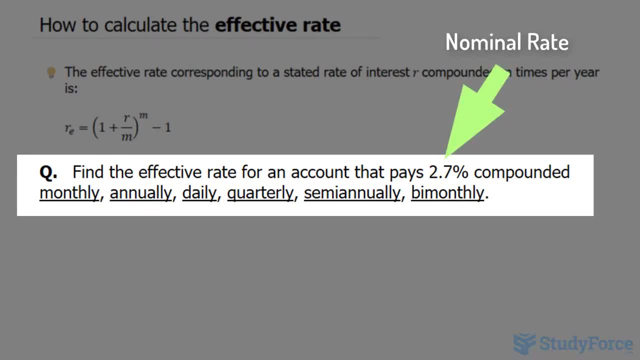 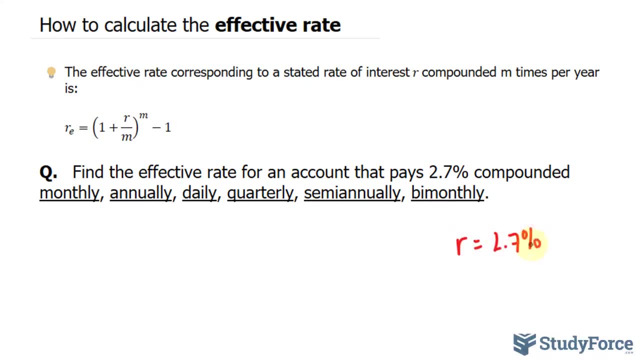 and we have to find out monthly, annually, daily, quarterly, semi-annually and bi-monthly. So R represents in our case 2.7%. We want to convert this as a decimal, so we divide this number by 100. 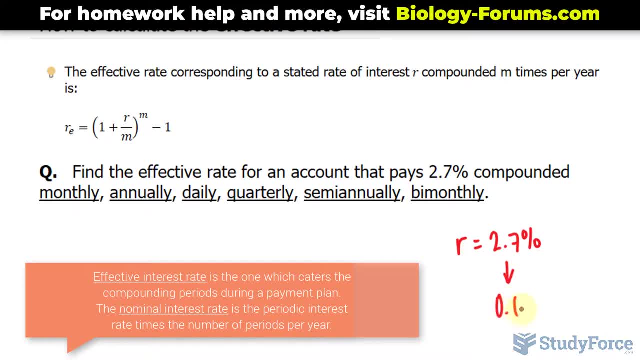 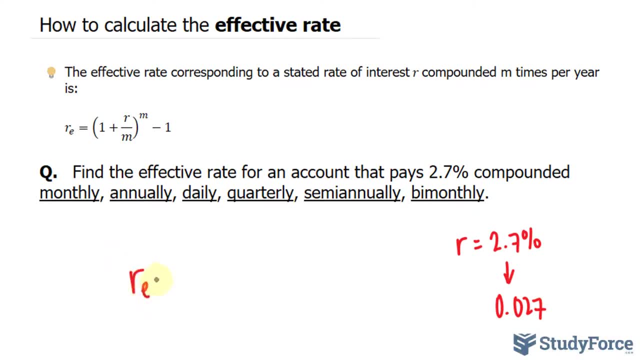 If we divide this by 100, we'll end up with 0.027.. So we just found our R and we can start substituting that into our formula. So the effective rate is equal to 1 plus 0.027 divided by m. 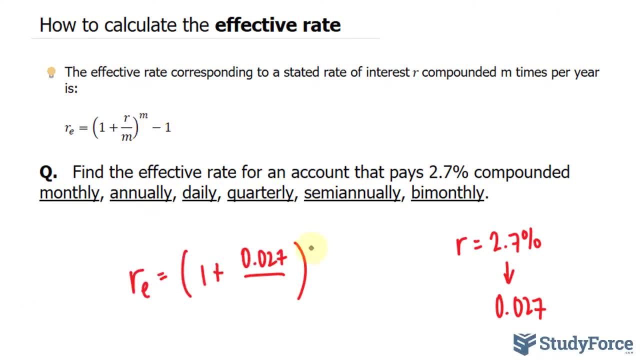 which we'll put in in a moment, This m, which we'll leave blank, minus 1.. Now m is determined by the words. In case we're using compounding monthly, your m value is simply 12, because there are 12 months in a year. 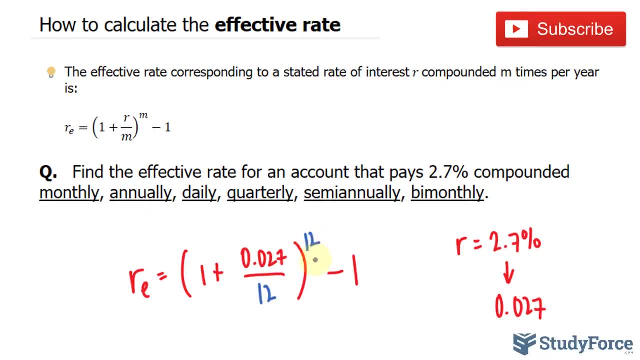 So it's always relative to one year, m is equal to 12.. Now, before I calculate this, I'll tell you what these numbers are. or the m is for the other five, For annually, m will be 1.. 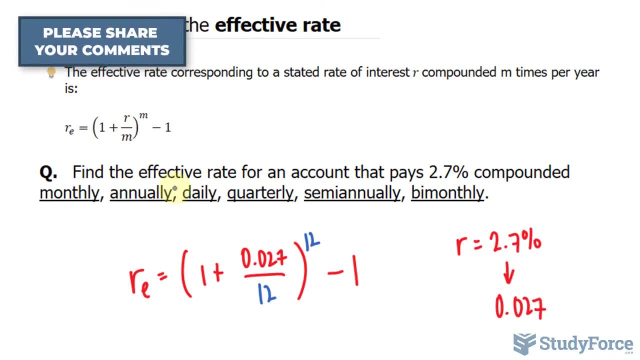 As a result, you should expect your effective rate and your nominal rate to be the exact same, So both. So this will come out as 2.7.. So here m is equal to 1.. For daily, we divide R by 365.. 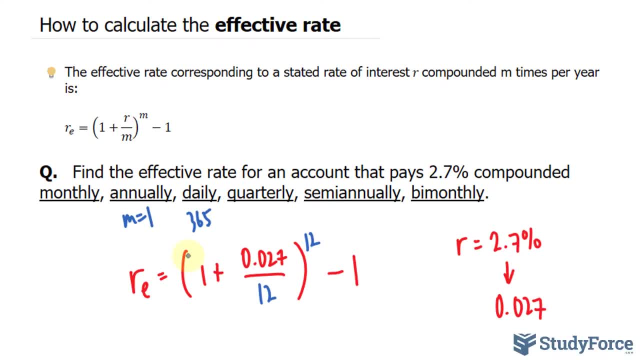 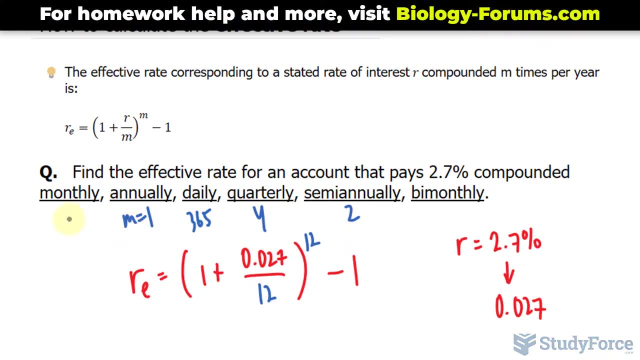 Quarterly, we divide by 4.. So we're dividing the year in quarters, which is 4.. Semi-annually: 2.. Bi-monthly means that we'll multiply the monthly, which we found to be 12, by 2,. 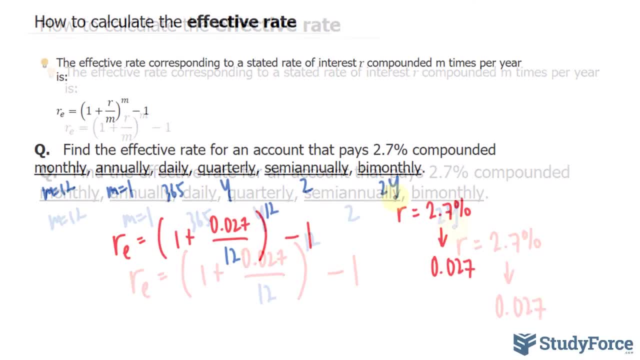 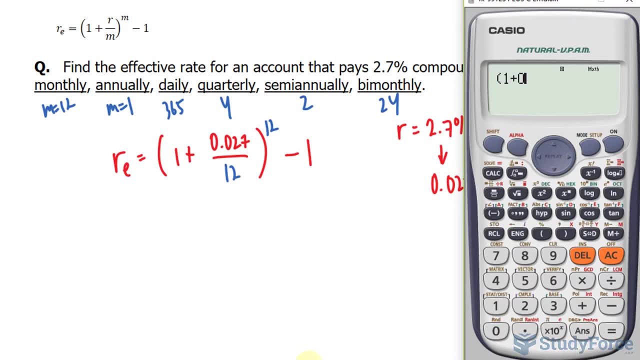 because it's happening two times a month. So we divide that by 24.. So let's go ahead and calculate the monthly. We have 1 plus 0.027 divided by 12.. Close the bracket. raise that to the power of 12 minus 1.. 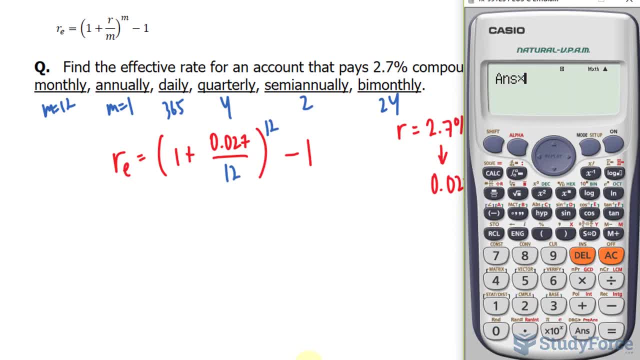 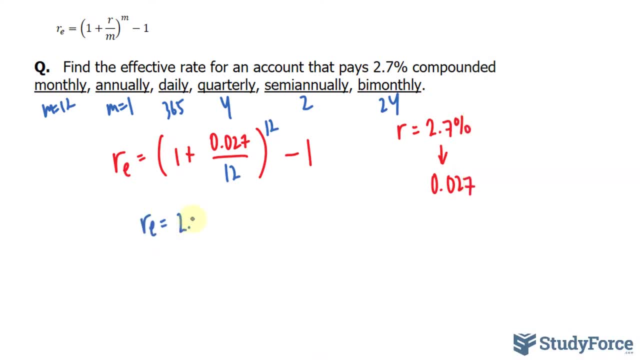 We end up with 0.027, and you want to convert this into a percentage, so you multiply by 100, 2.73%, So the effective rate is approximately 2.73%. Let's see how this changes if we make m equal to 1.. 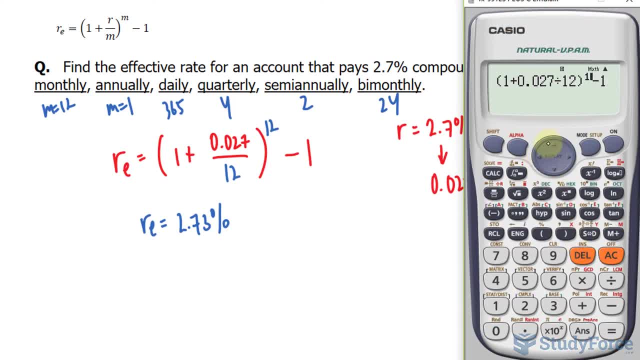 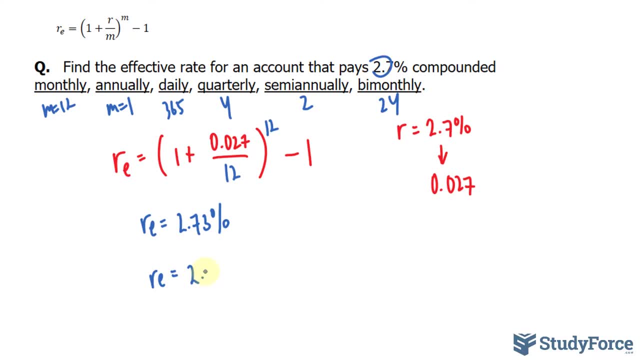 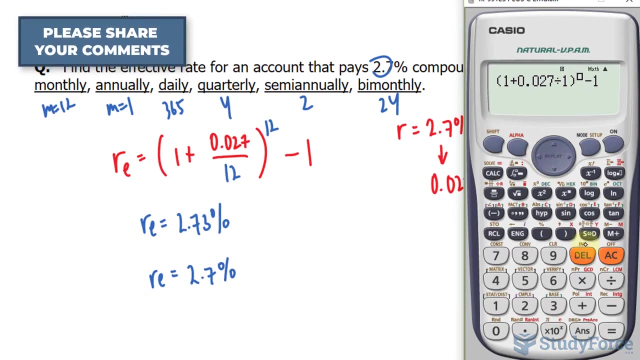 So, going back here, I'll replace this 12 with a 1, and that with a 1. And we end up with so the same percentage. we started with 2.7%. What about daily? We'll switch this to 365,.